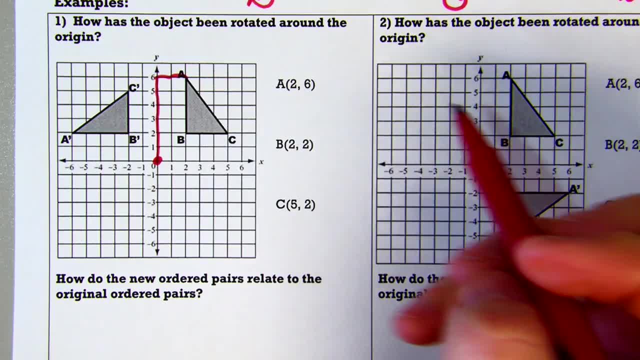 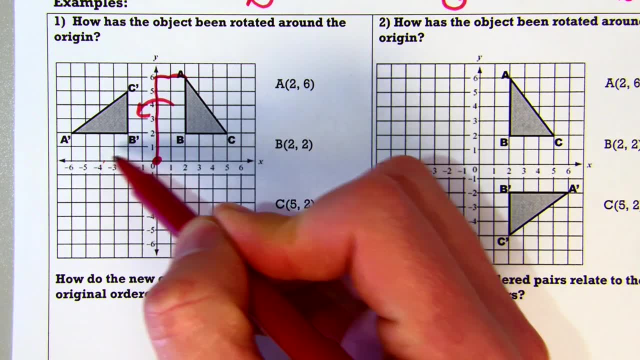 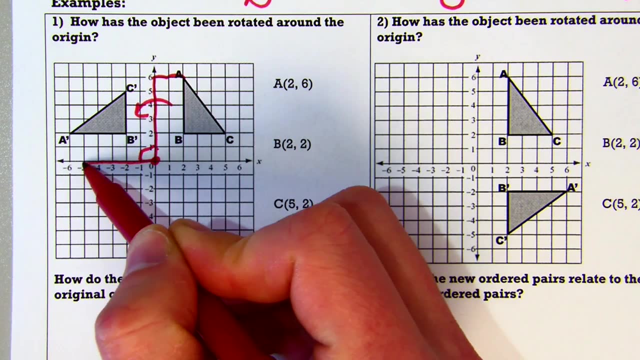 five, six. Because I'm going, in this case counterclockwise- this arm is going to kind of swing down here And it's going to create a 90 degree angle- And because I came down six, I'm going to go over six: One, two, three, four, five, six. And I'm going to go because 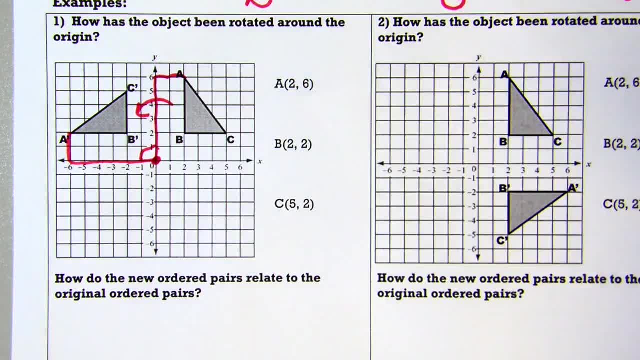 I came over two. I'm going to go up And I'm going to go down six And I'm going to go up two. So you can kind of see how this bar just kind of swung right down And our A goes to our A prime over here. 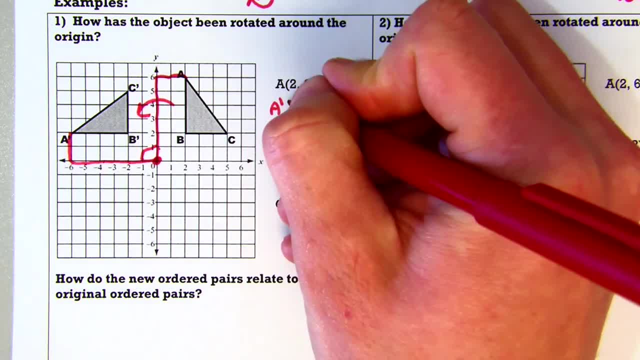 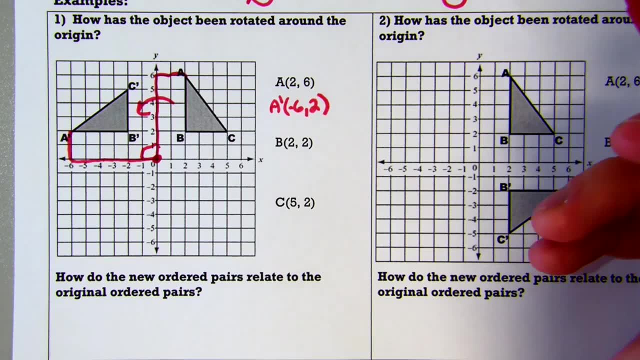 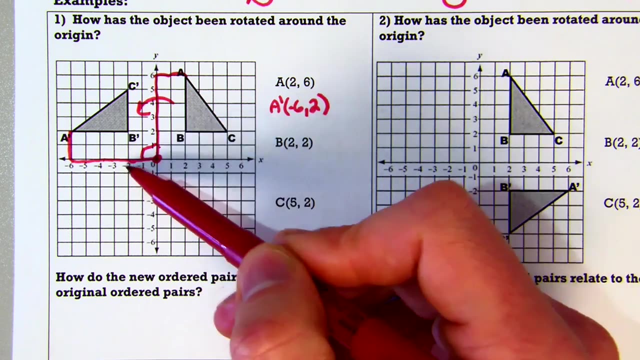 And so our A prime turns out to be a negative six two. Now let's go ahead and see what happens with B. So B goes over two, down two, which means we're going to go over two and then up two. That bar is going to kind of swing down, And our B prime turns out to be 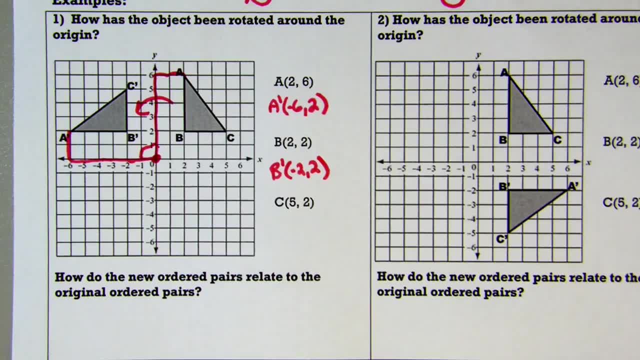 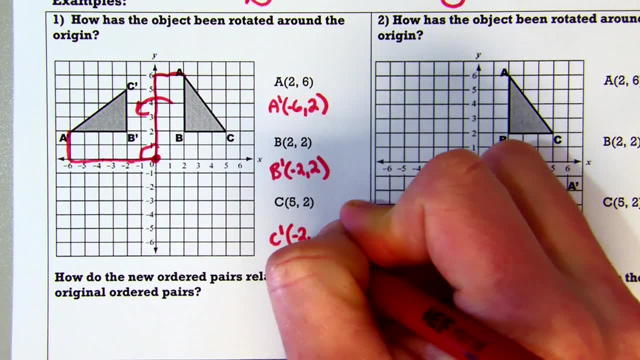 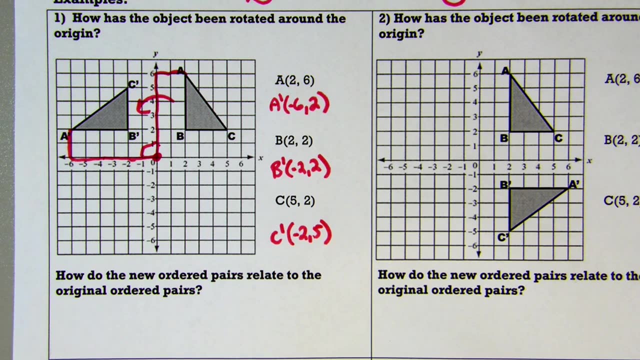 a negative 2, 2, and then, if we look at our c prime, our coordinate, we have a negative 2 and a 5.. So now let's go ahead and compare our x and our y. all right, Our original x and our y. 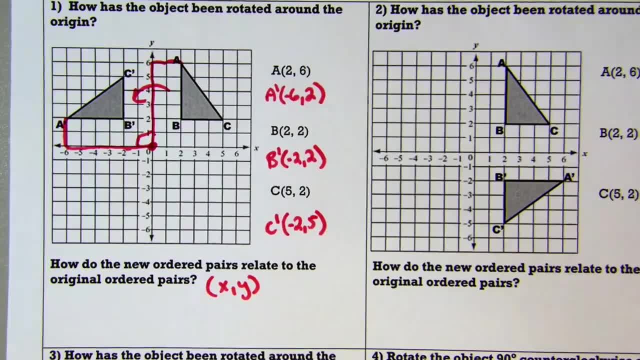 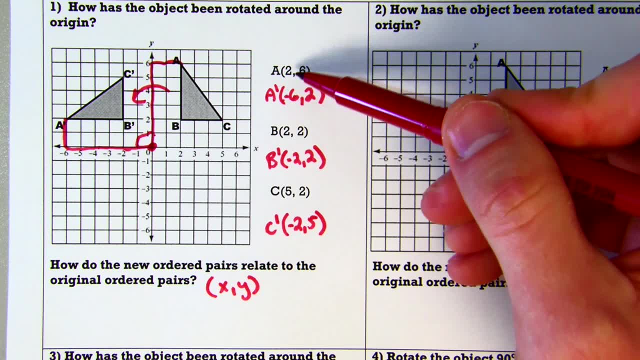 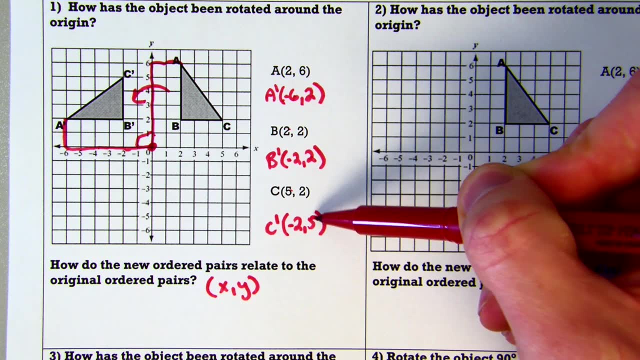 we can go ahead and write here. that's our original. and now, if we look at what happens to it, notice how every single time our y turns into our x and it actually becomes negative. And then each time our x just turns into our y, so 2 becomes 2, 2 to 2, 5, 5.. Now look at our y. 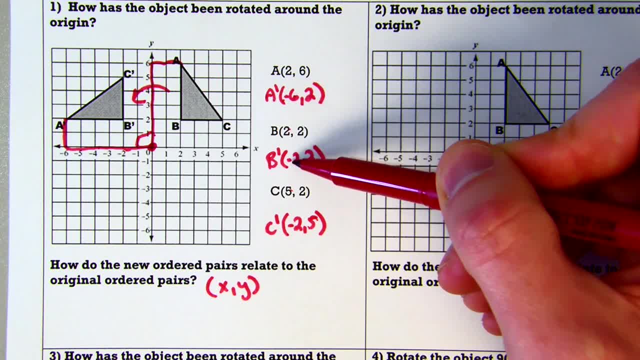 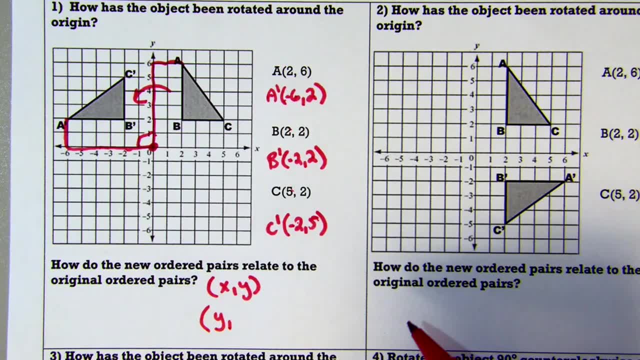 it's going to turn to our x, but it's going to be negative. 6, goes to negative 6, 2 goes to negative, 2, 2 goes to negative 2.. So our new ordered pair, our y, is coming over here and then our x is. 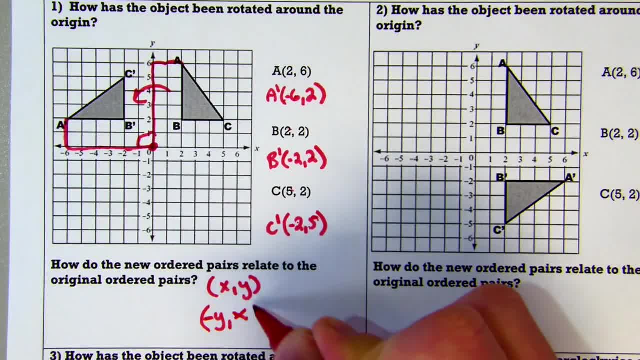 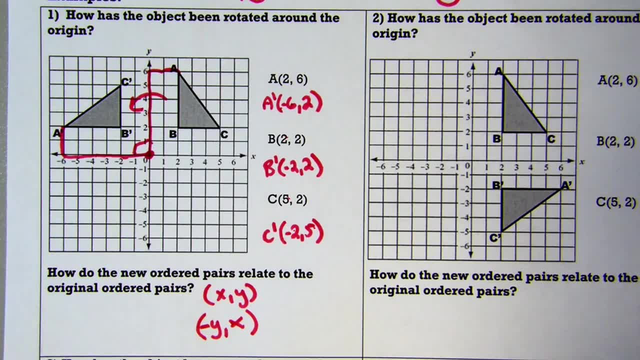 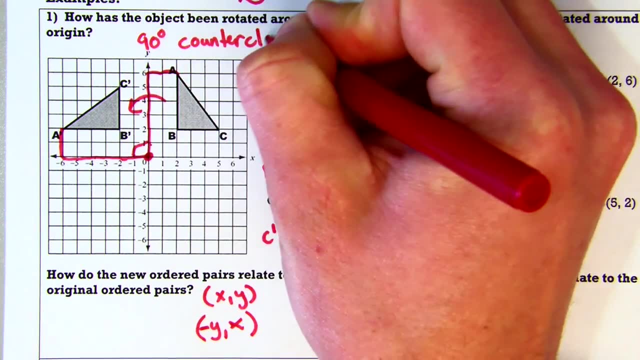 I'm sorry. and then it's turning negative and then our x is staying the same. So our new ordered pair is negative yx for an object That has a- we could say- 90 degree counterclockwise. All right, let's go ahead and look at number two. 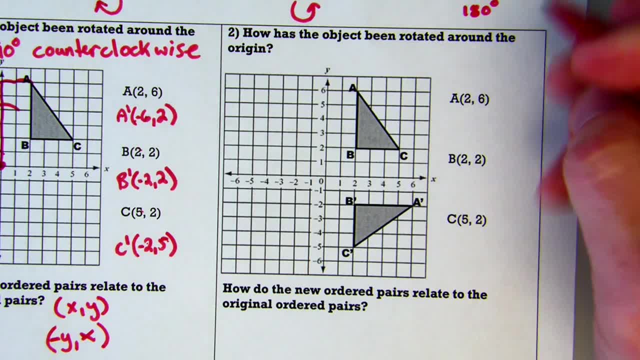 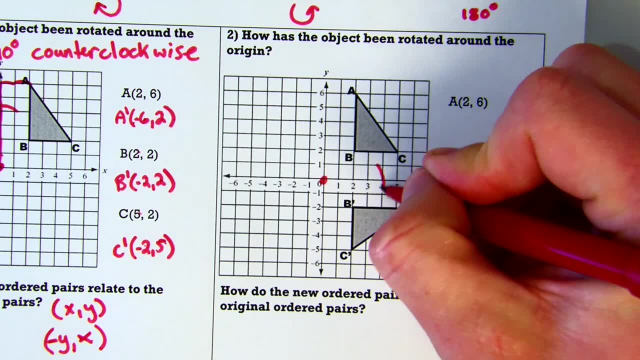 How has the object been rotated around the origin? So the first thing I want to go ahead and look at is we're going from our letters to our prime letters. So here's our rotation direction. So in this case again, we are going clockwise. 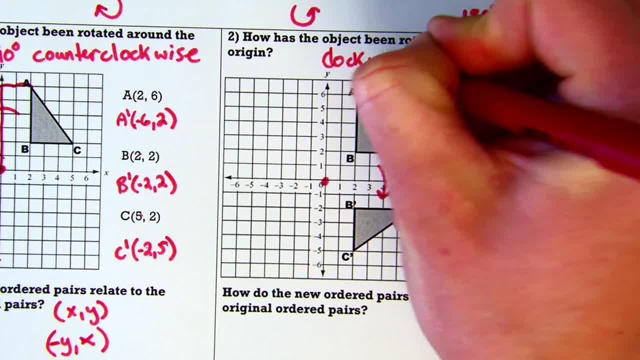 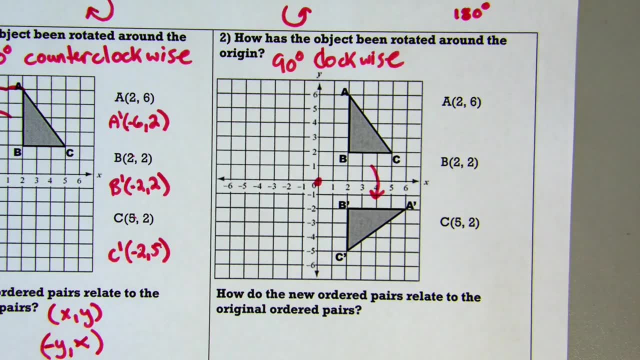 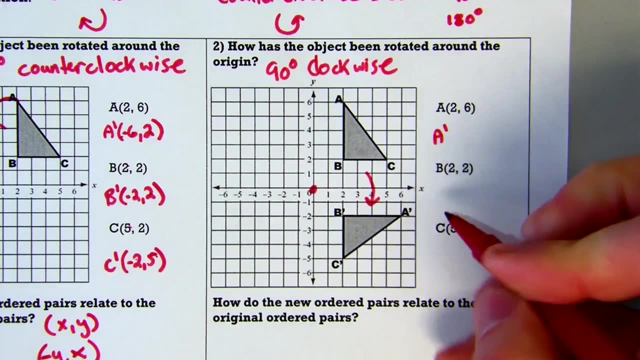 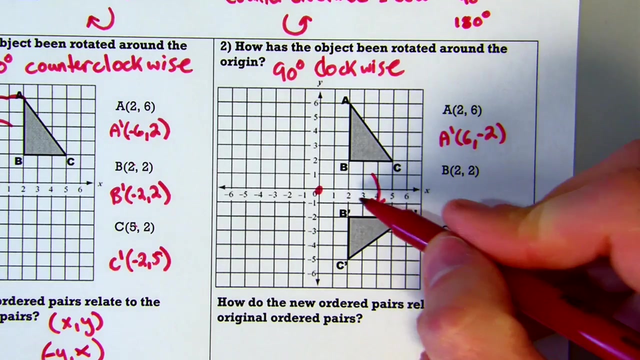 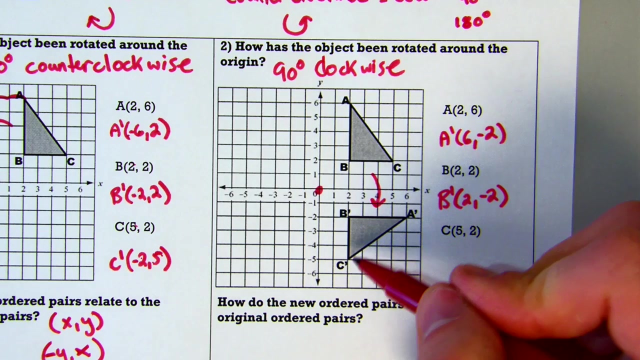 And our clockwise rotation is actually 90 degrees because we went over one quadrant. Now let's go ahead and write our new ordered pairs. Our a prime is 6, negative 2.. Our b prime is 2, negative 2.. And our c prime is our 2, negative 5.. 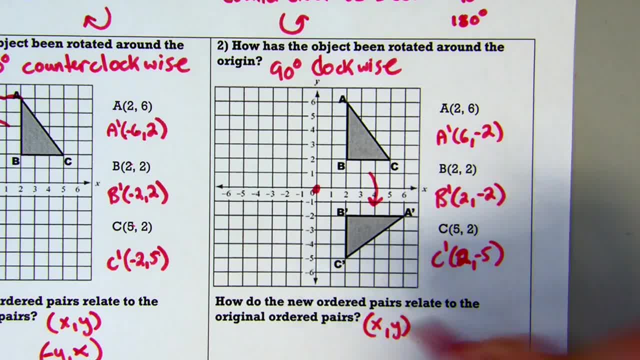 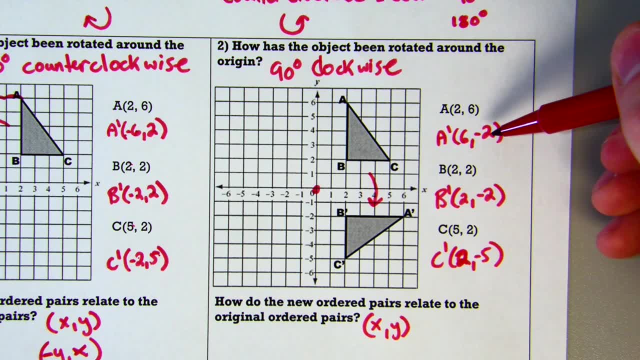 So we talk about our original x, y. Now we're going to go ahead and take a look at what happens to x, x over here at our 2, 6,. 2 goes over to our y spot and it turns negative. 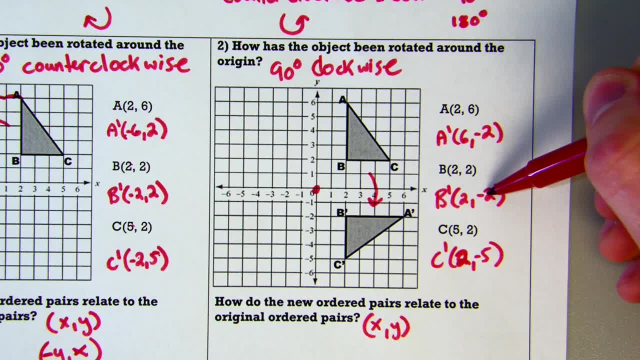 Let's check and see if it's the same way. 2 goes over to y and turns negative. 5 goes over to x. 5 goes over to y and turns negative. 5 goes over to y and turns negative. 5 goes over to y and turns negative. 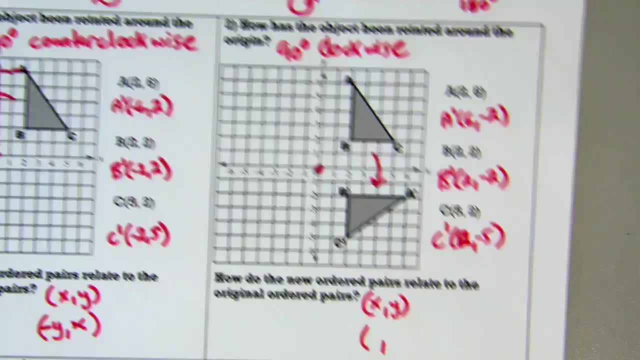 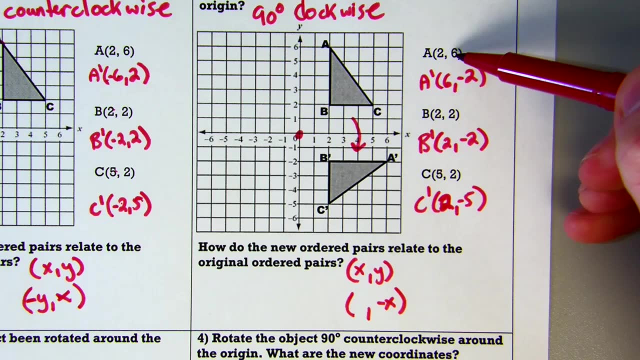 5 goes over to x. 5 goes over to x. 5 goes over to x, to Y and turns negative. so our new order pair is going to have it be a negative X over. here and now. let's go ahead and look at what happens to our Y. our Y just. 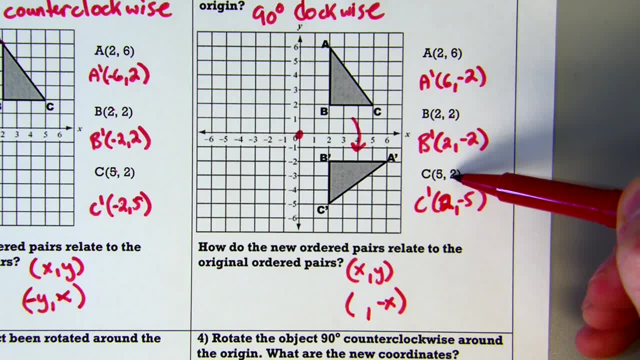 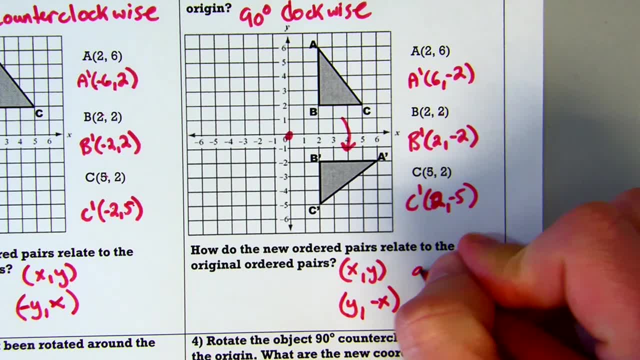 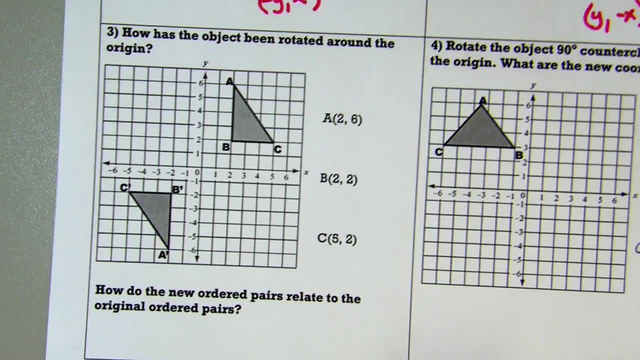 goes over X doesn't change, Y goes over to X doesn't change, and our Y goes over X doesn't change. so our new order pair is Y negative X, and again it is a 90 degree clockwise. so number three we have. how has the object been rotated around? 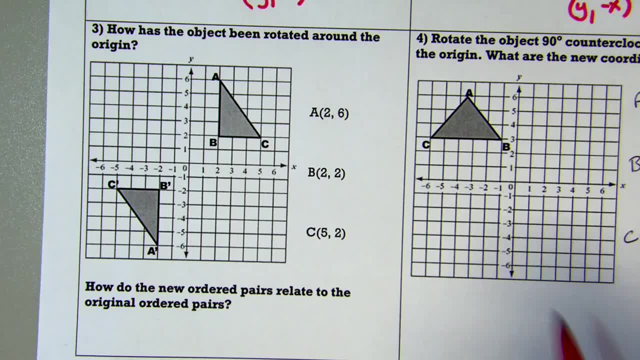 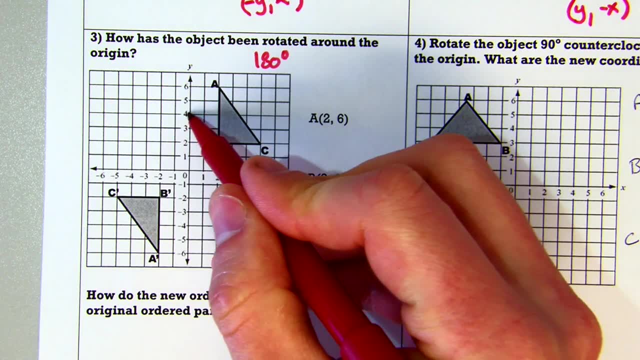 the origin, okay, and notice how it's moved to cordon or two quadrants, so we know that there has been a 180 degrees. okay, now, if we want to go this way, we can or we can go this way. it doesn't matter which way we go, so it is either a 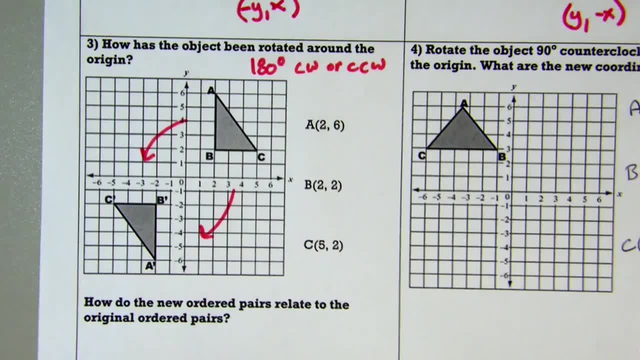 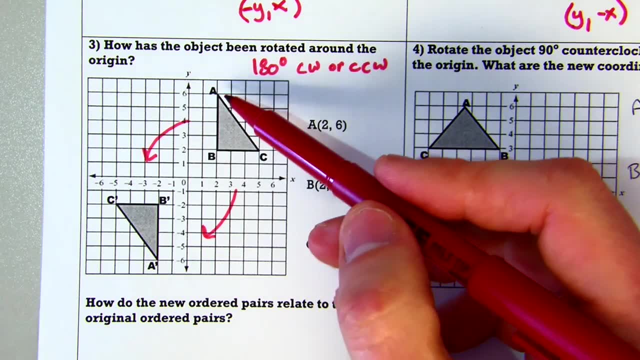 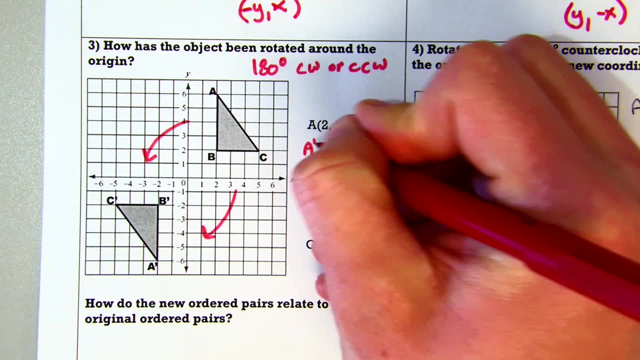 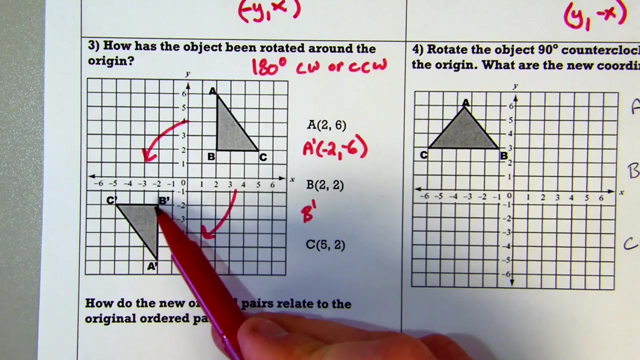 clockwise or counterclockwise. either one we want it to be is fine. let's go ahead and look at our new coordinates. here we have our B, that's whatever they actually are. a new coordinate is a negative two, so a prime is negative, two negative six. our B prime turns out to be a negative two negative. 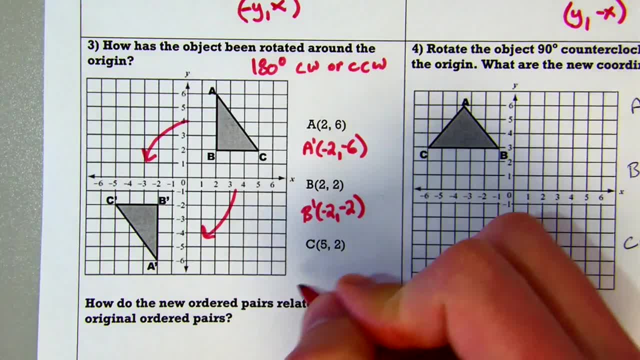 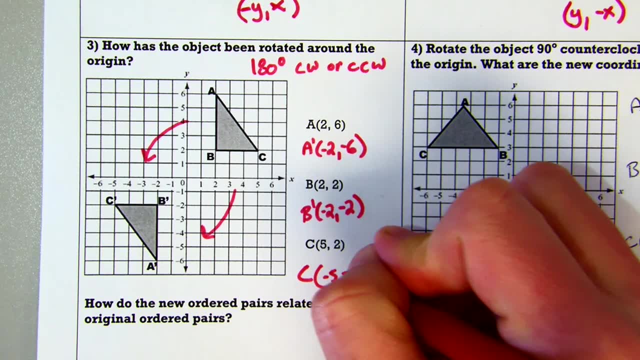 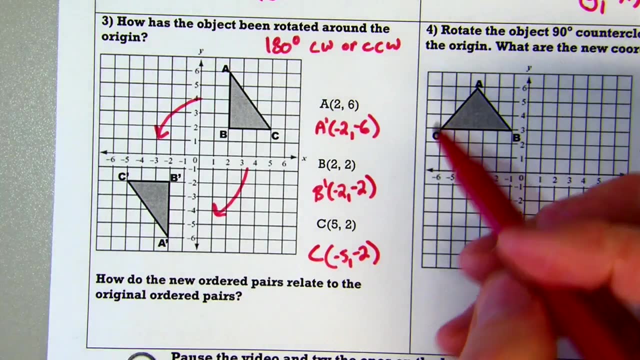 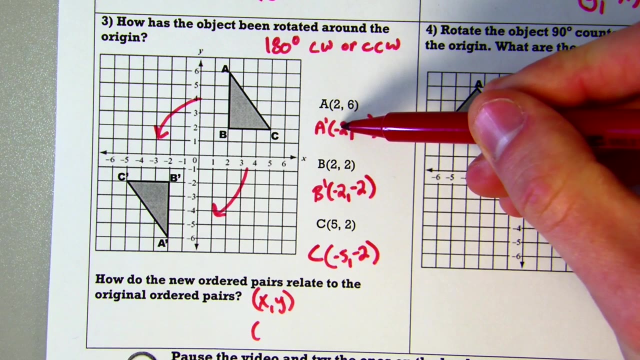 two and our C prime turns out to be negative five negative two. so now, if I want to go ahead and compare what happens to each of them, alright, I noticed that my start with that XY start with my X. my X stays the same but turns negative. up here, my X stays the same but turns negative right. 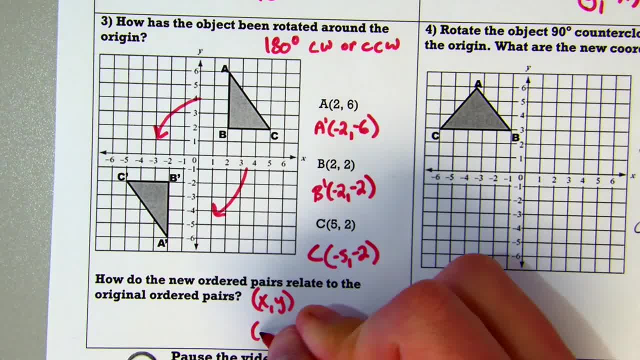 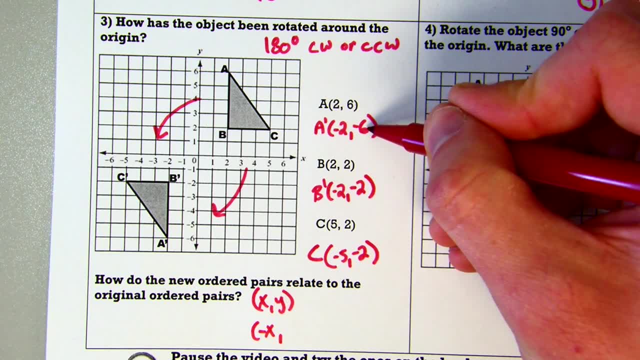 there. and then my X stays the same but turns negative right there. so X just turns into a negative X. with that rotation, my Y stays in the same spot, it turns negative, 2 turns to negative 2, and then 2 turns to negative 2.. So Y again. 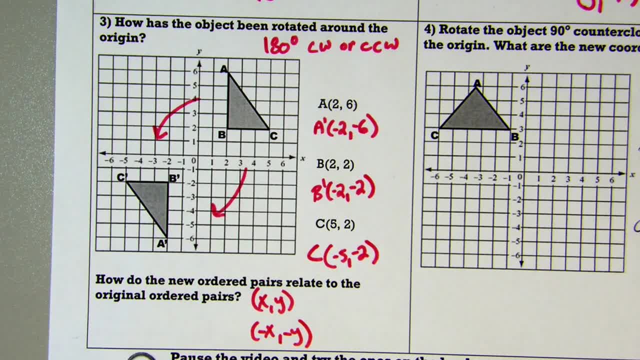 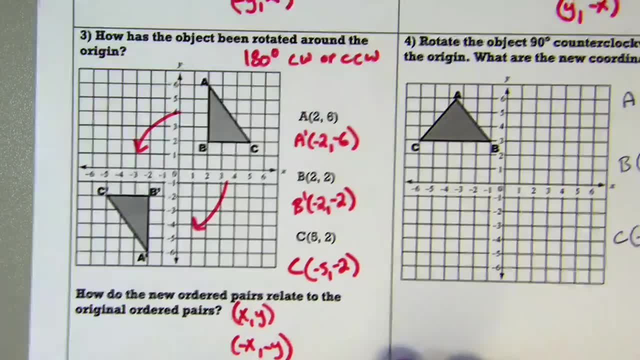 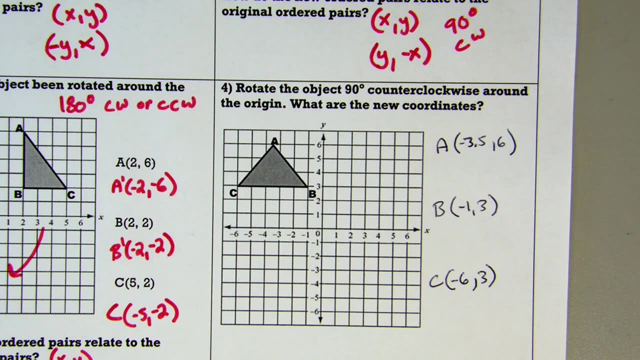 stays in the same spot but turns negative. So my new order pair relates is negative X and negative Y. That's how it relates to my original. Alright, let's go ahead and look at number 4. now. Number 4, we've got a rotation of 90 degrees. 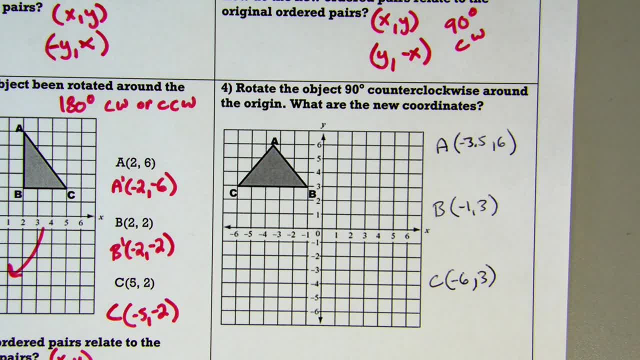 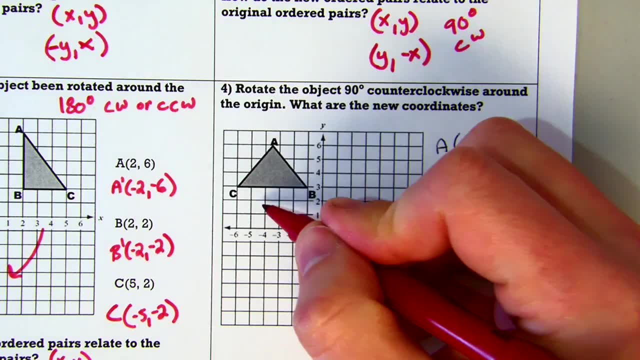 counterclockwise, around the origin. So what is our new coordinate? So this time we're actually looking what the new coordinates are. So again, it's around the origin and I know that it's counterclockwise, so it's going to be. 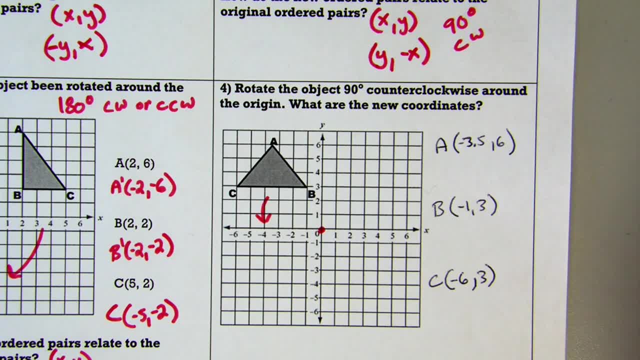 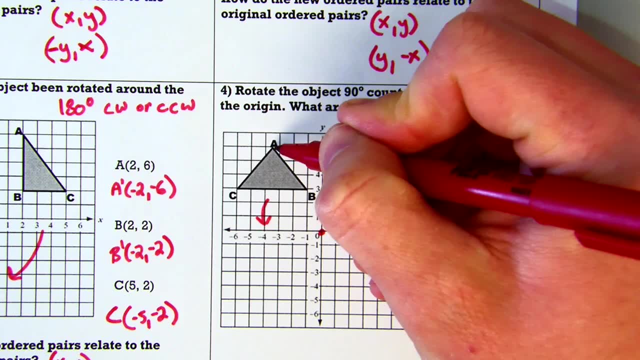 going this way. So the first, and it actually goes 90 degrees as well. So the first thing I want to do is take my A here and notice how it goes. it looks like it's at about three and a half two. So we're gonna go, let's start, we go over. 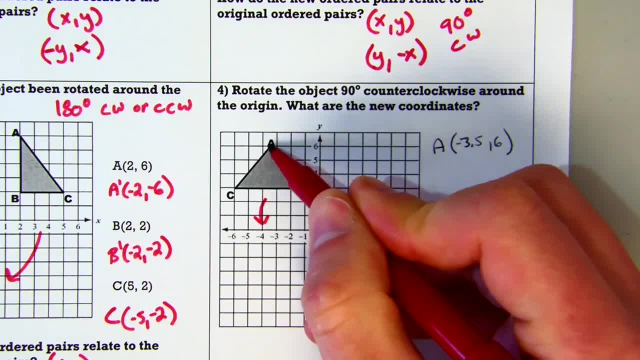 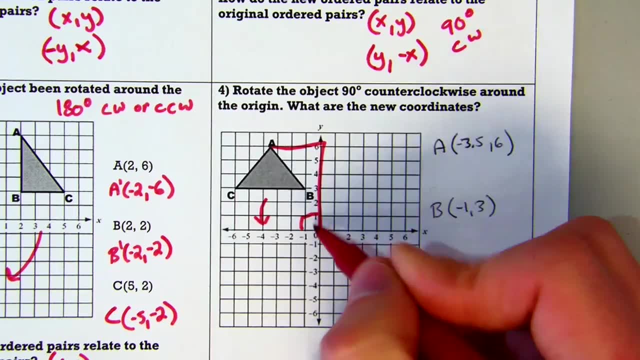 three and a half and then down six. So let's draw this line here. and then we wanted to create a 90 degree. So this bar is completely negative. So I want to create a 90 degree, So this bar is kind of of just dropping down. so we're going to be going over six, and then we're going to be going over 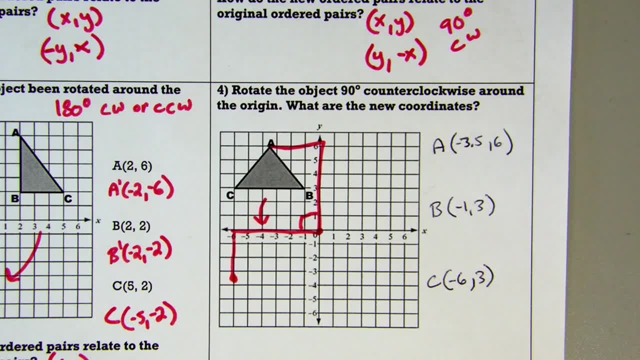 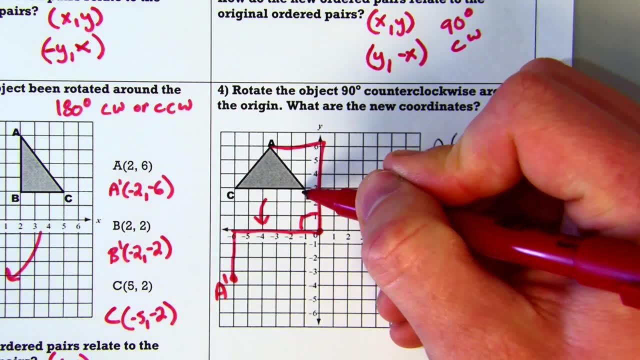 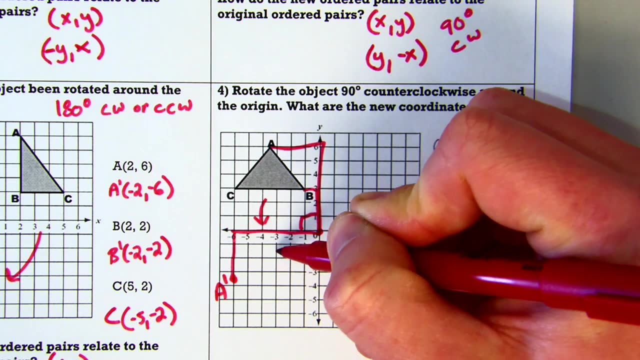 three and a half and right there between that three, negative three and negative four. that is my a prime. okay, if i look at my b looks like i come over one and then down three. so again, is that bar that's just dropping down? it's rotating this way. so i go over three and down one. that's my. 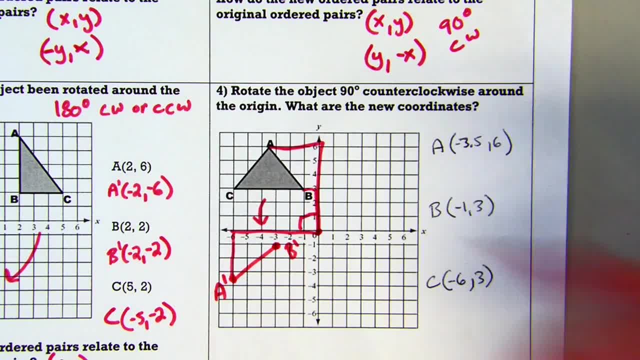 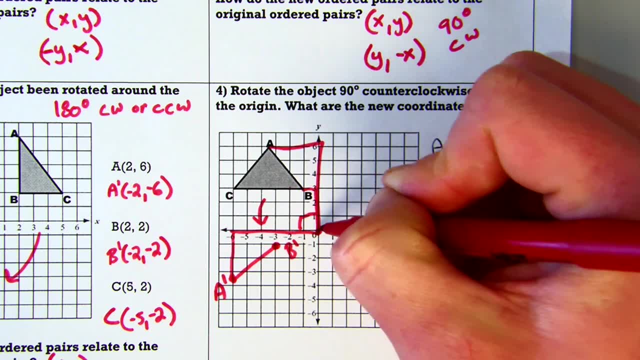 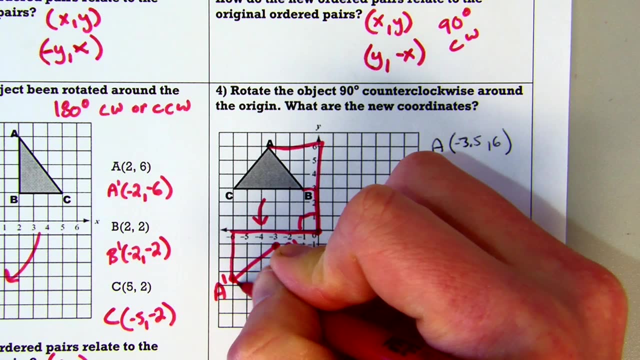 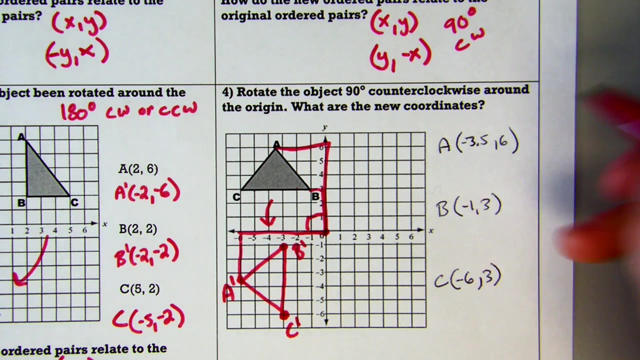 b prime. go ahead and connect those two, all right. and then c, we have one, two, three, four, five, six comes over six, down three, which means i'm going to go down three over six and i get my c prime. go ahead and connect those two, all right. now i'm going to go ahead and write my new coordinates. my a prime is over negative six. 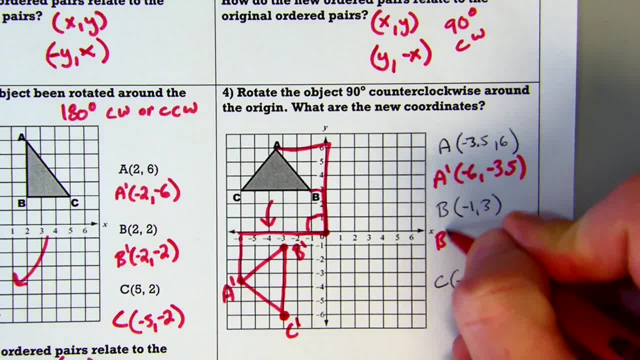 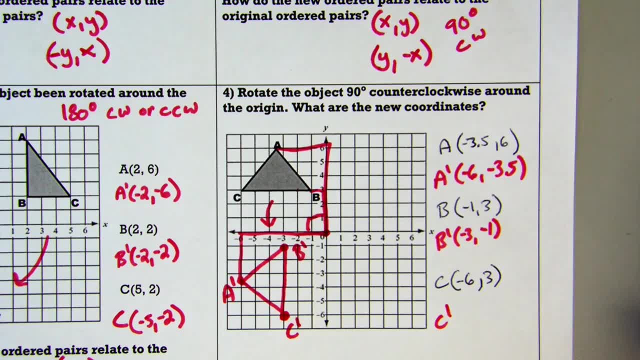 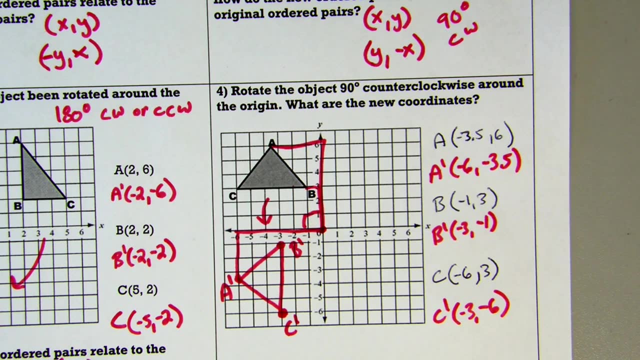 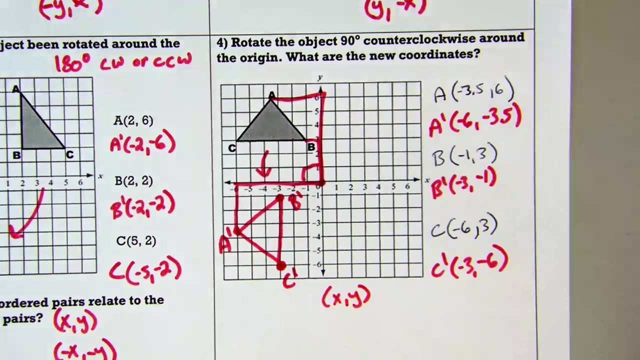 and then negative three and a half. my b prime is over negative three, down negative one, and my c prime is over negative three and down negative six. there's my new coordinates now. now let's go ahead and check to see what happens. okay, if i have a, x, y, i notice that my x moves over to my y. up here, x moves over to my y. 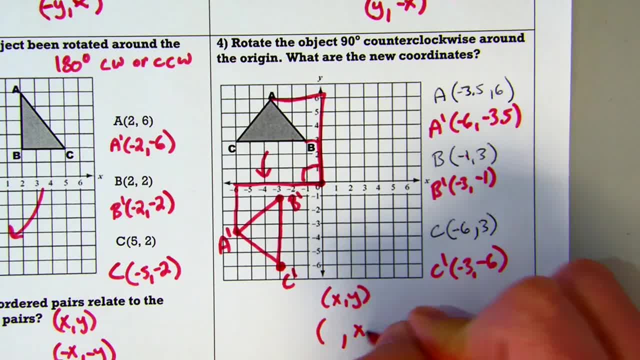 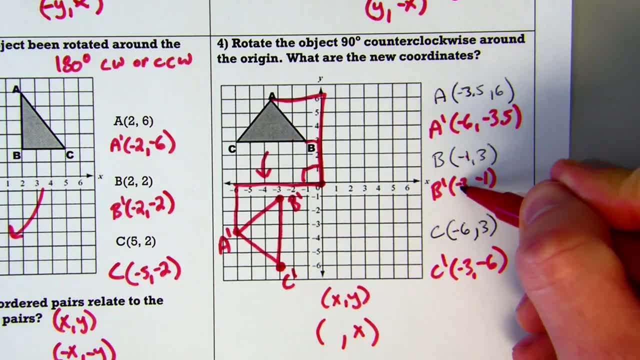 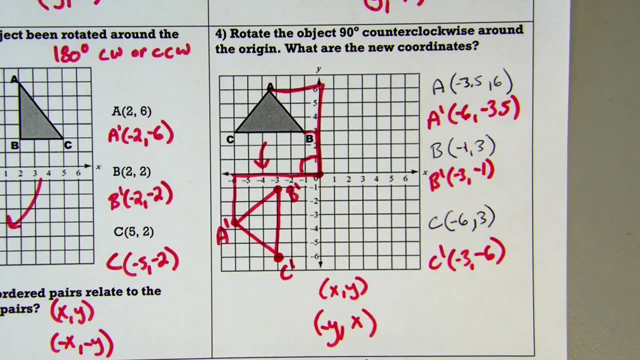 x moves over to my y. so my new coordinate is just going to move my x over there. now my y moves over to my x spot but turns negative. moves over to my x, turns negative. moves over to x, turns negative. so i'm going to do a negative y there. so those are our four examples for 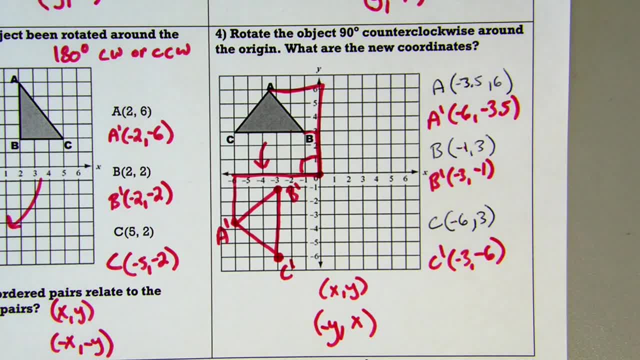 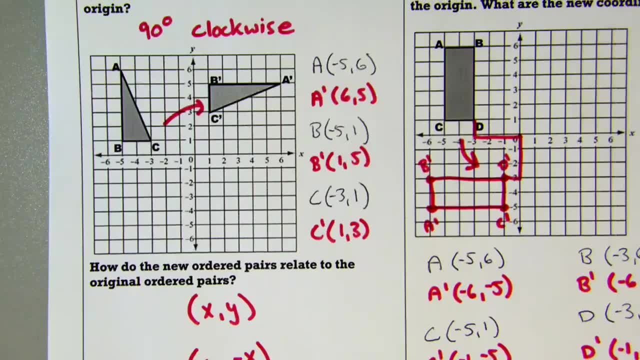 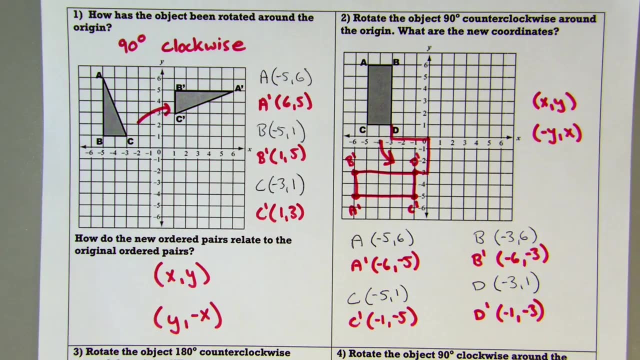 rotating. what i'd like to go ahead and do now is pause your video. go ahead and try the four examples. all right, let's take a look at how we did here. all right, our first one we have. how has the object been rotated around the origin? we should have set a 90 degrees and you should have had a. 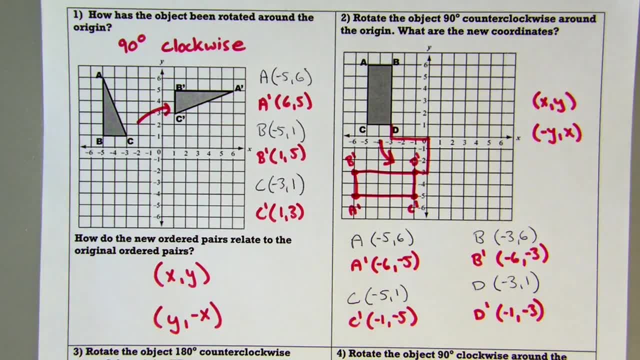 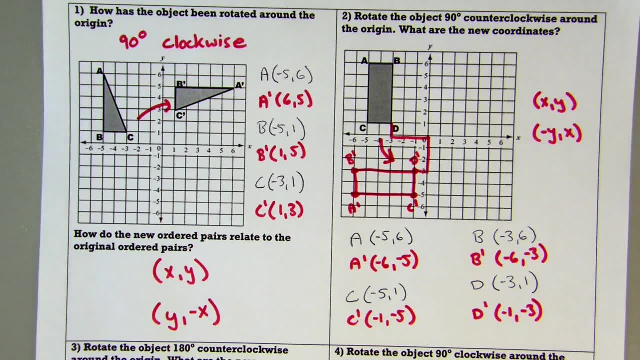 x turns to negative x in the y spot and my y slides over to my x, so you should have gotten a new ordered pair of y negative x. number two: you have to rotate the object 90 degrees counterclockwise around the origin. what are the new coordinates? 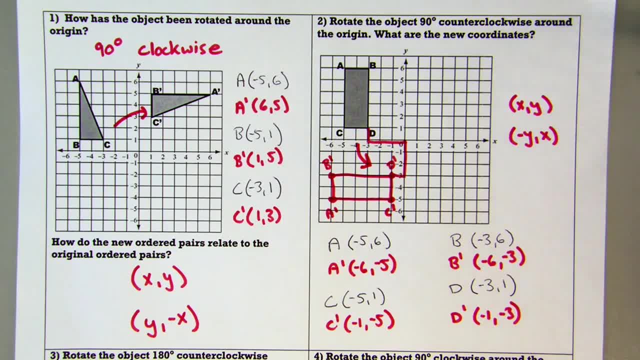 okay, so notice how I bring it counterclockwise right here. make sure you write all of your prime origins here and you should have figured out that- sorry, all your prime coordinates. and you should have figured out that your new ordered pair, instead of XY, should be negative Y, X. number three: rotate the. 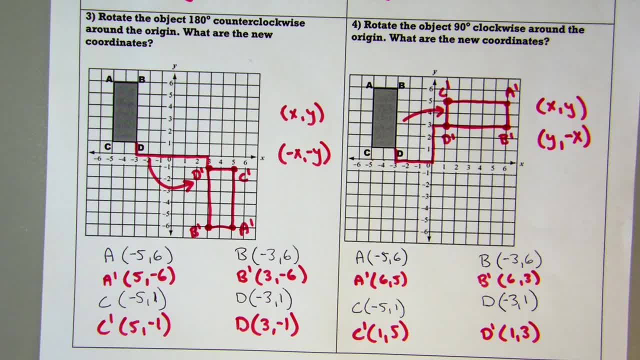 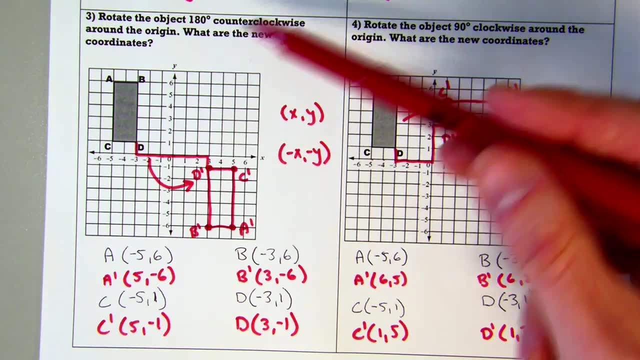 object: 180 degrees, counterclockwise, around the origin. what are the new coordinates? so again, when you go 180 degrees removing two quadrants, you can go counterclockwise or clockwise. this one says counterclockwise, so we want to make sure we follow that and you should get an answer of XY turns into a. 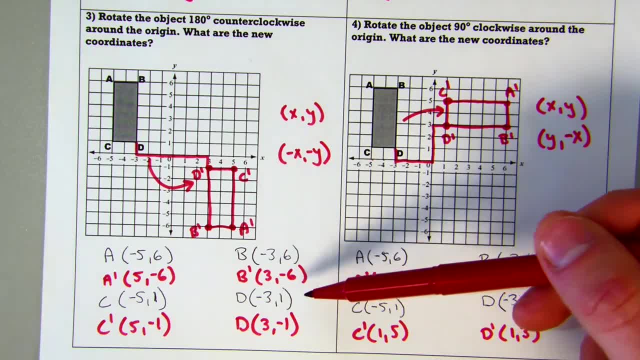 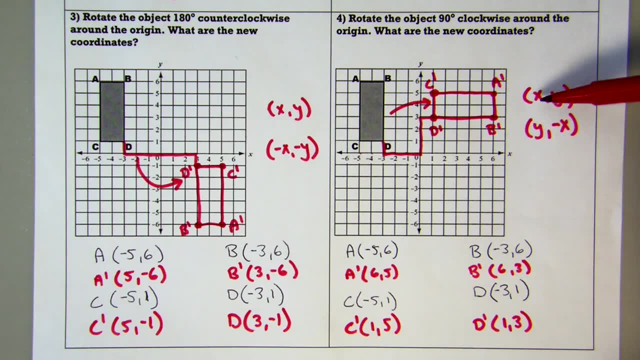 negative X, negative Y. and there's your coordinates, if you didn't get the right answer to compare them. and number four, we have- rotate the object 90 degrees clockwise- should have gotten an answer of XY turns into Y, negative X. and again there are your prime coordinates so that you can compare to make sure. you, you. 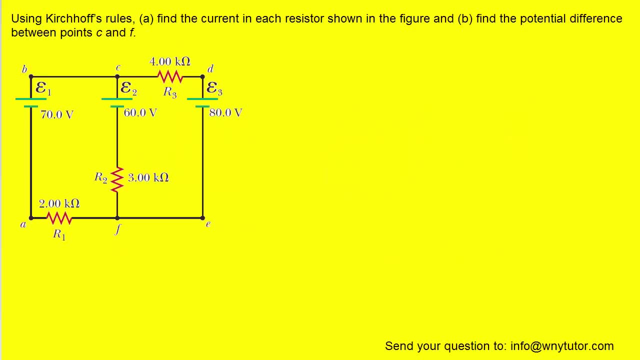 If you haven't done so yet, please pause the video and try to answer the question on your own before listening on. Our first step in solving this question is to draw in the currents, and when we draw in those currents, we have to make sure that we do it for each branch of the 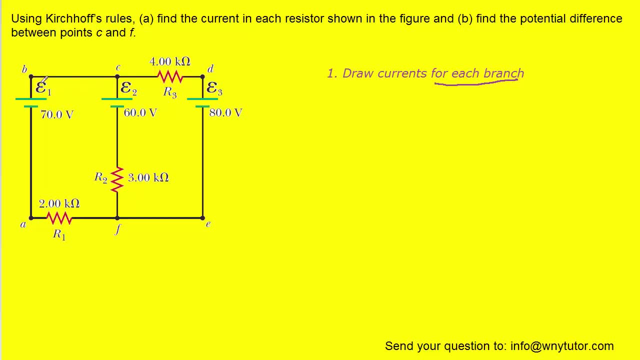 circuit. So let's take a look at how we could do that. We'll head on over to the first battery that's marked E1. right here, and typically when you draw a current you, you draw it so that it projects away from the larger terminal of the battery. You can see there's a large terminal. 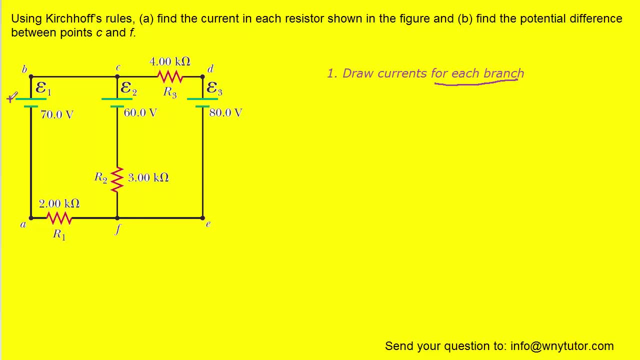 here and then a smaller terminal. here, It's common to label the large terminal with a positive sign and the smaller terminal with a negative sign, and again, current typically, though not always typically, exits from the positive terminal of the battery, and so what we can do is project an arrow. 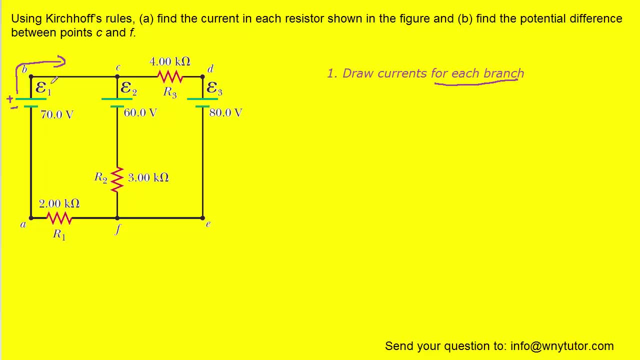 that's heading in this direction and since they've labeled this E1, we can call the current I1.. Similarly, if we come over here and we draw in the current E1, we can call the current I1.. Here to this battery, it's marked E3.. The larger terminal is the positive terminal, The smaller one. 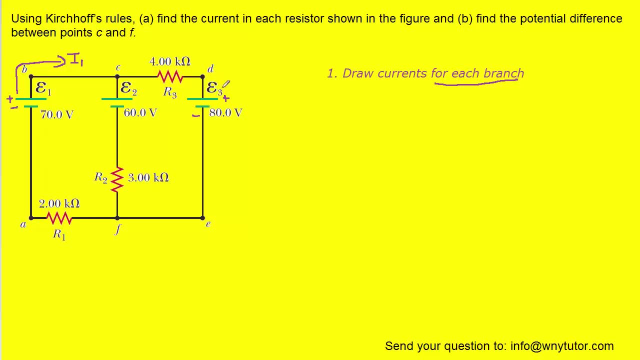 is negative, We project the current away from the positive terminal typically, so we'll draw an arrow going in this direction and we can label that current I3. and then we come to this branch of the circuit where we have the E2 battery and it might be tempting based on what we've said so far.